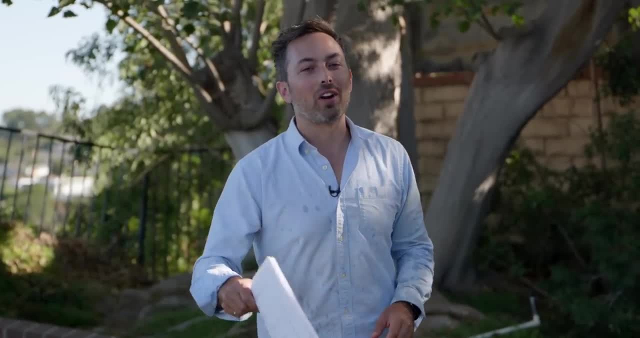 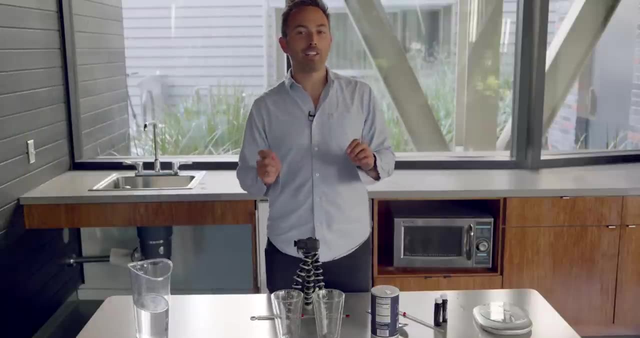 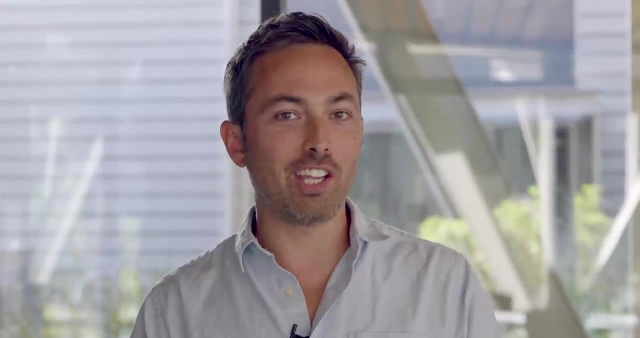 So we will find out what it is after we explore the second perplexing physics problem. Consider this: If you put identical ice cubes in a cup of fresh water and a cup of salt water, which ice cube will melt first? Again, you can register your prediction by answering. 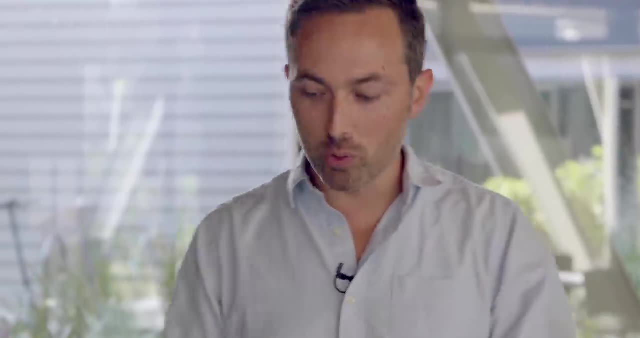 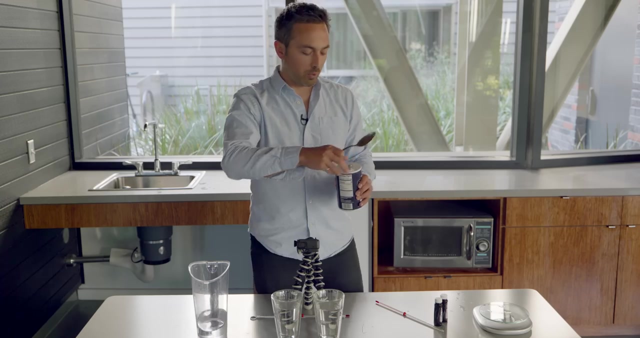 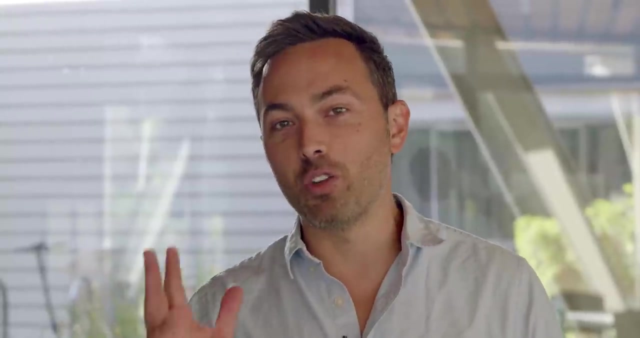 the poll here. Now, as you're thinking about that, I want to show you the setup. Okay, so here I have regular fresh water. I'm just going to fill up each cup. Then I'm going to add about a tablespoon of salt into this cup on the right. Now, if you know a bit about chemistry, you may recognize. 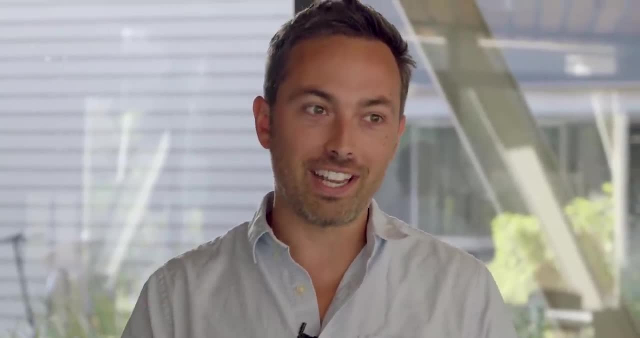 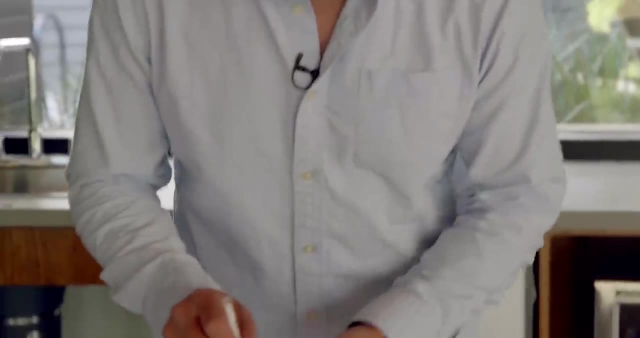 that adding sodium chloride to water actually takes energy, And so it lowers the temperature of this solution by a little bit. So I've got a thermometer just to check And I'm going to let this solution sit here for a while so that it comes back up. 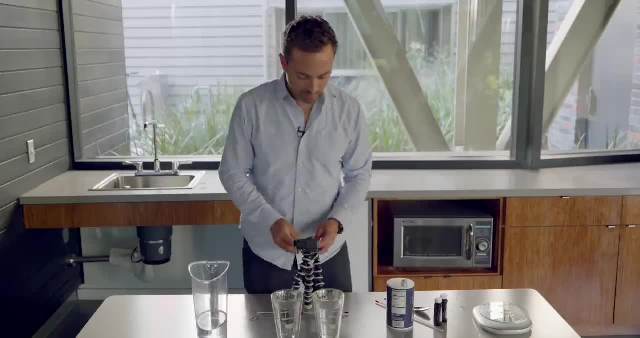 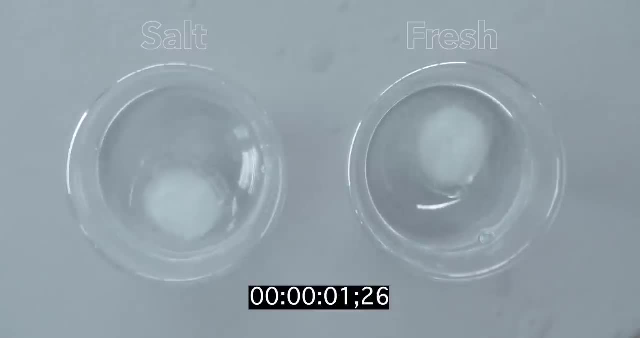 Okay, have you made your prediction? Let's put these ice cubes in in three, two, one And they're off Watching ice cubes melt. Isn't this entertaining YouTube? It has only been about a minute, but already I can tell that the ice cube in the fresh water. 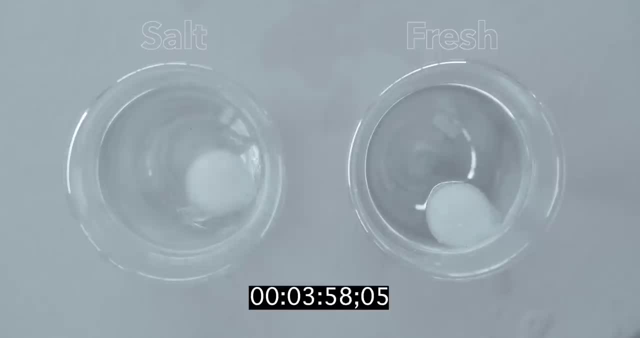 is melting faster than the ice cube in the salt water. How does that make any sense? I mean, we put salt on the roads to melt ice faster, So why isn't this ice cube melting as fast as the one in fresh water? Well, that is what I'm going to explain, But first, 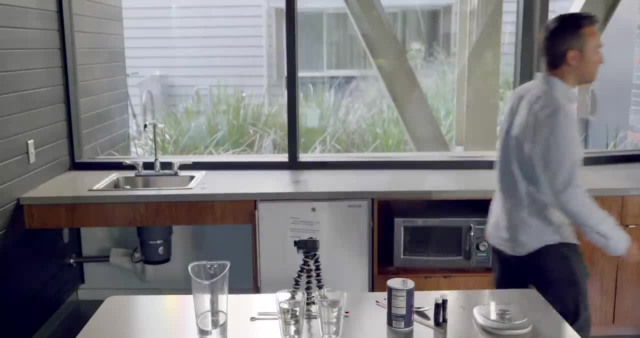 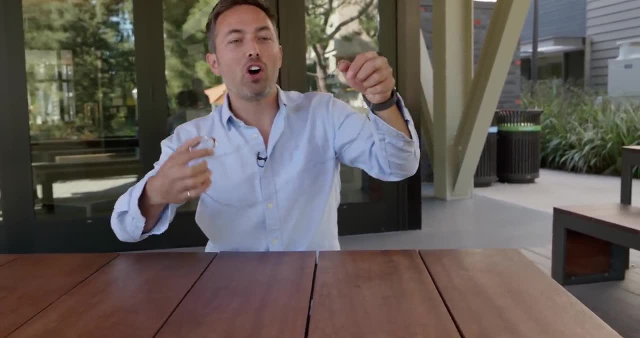 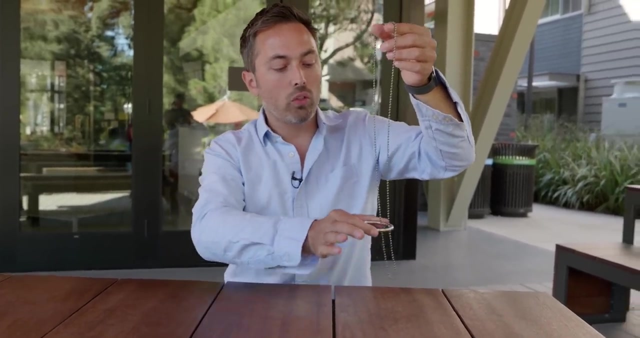 let's go to the third perplexing physics problem. Okay, here I have a metal ring and a closed loop of chain, And I'm going to do this all in one take. so you know that I'm not playing any tricks. So what I'm going to do is dangle the chain and then hold the ring. 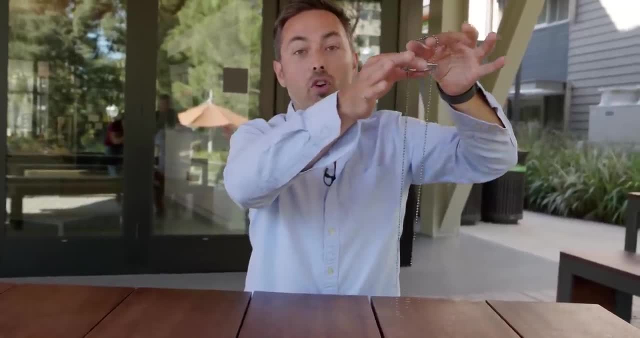 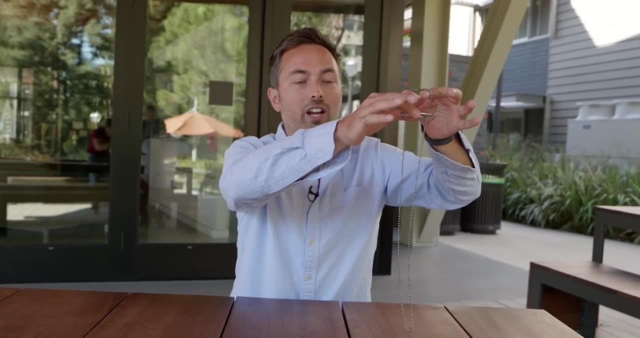 over it, like so, And then I'm going to drop the ring And exactly what you expect happens: The ring just falls off this chain. And, of course, how could anything else possibly happen? Because, well, it's a closed loop of chain and a closed 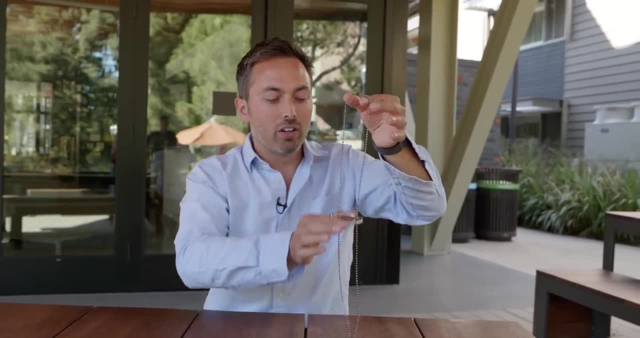 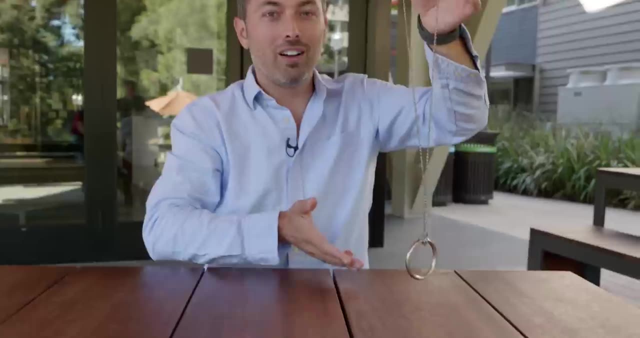 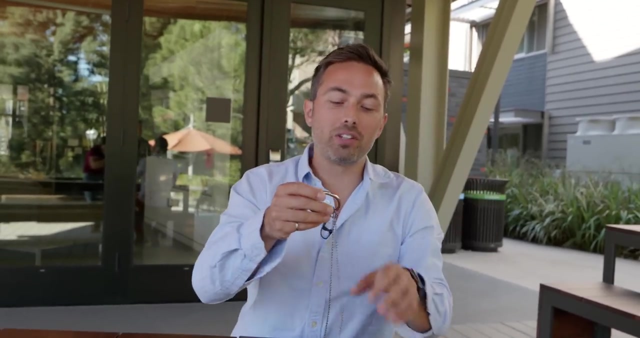 ring, But if you think about it really hard, you can get the ring to stick on the chain. Have a look at that. So how does this work? I think we're going to have to go to some slow-mo footage to really see what's going on. 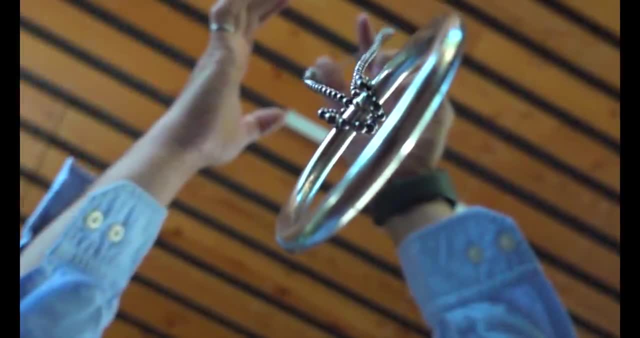 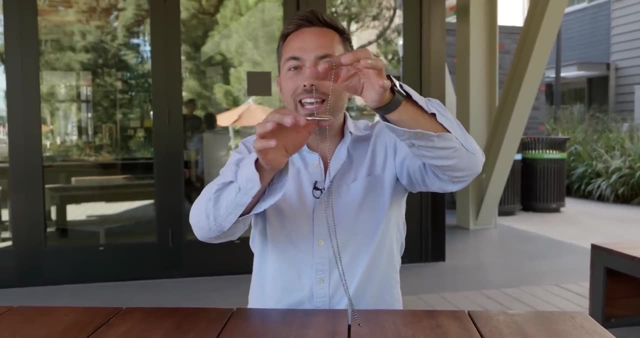 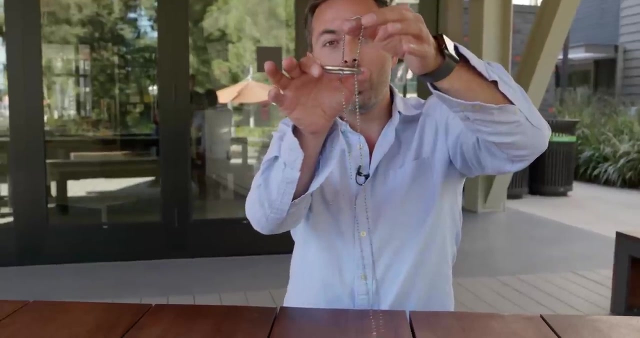 Now I'll let you in on the secret. When you want the ring to stick on the chain, the key is to let it go on one side before the other side. So I'm going to let it go with my thumb first and it'll just sort of slide off my finger. And by doing that 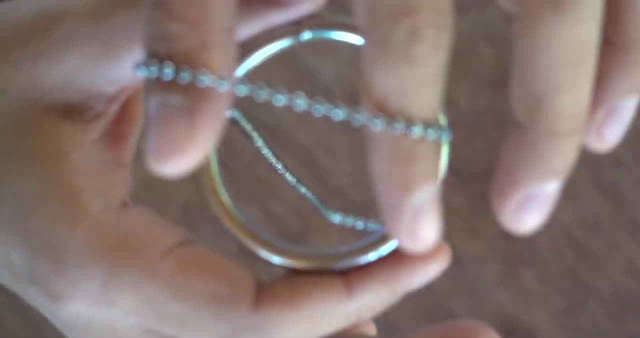 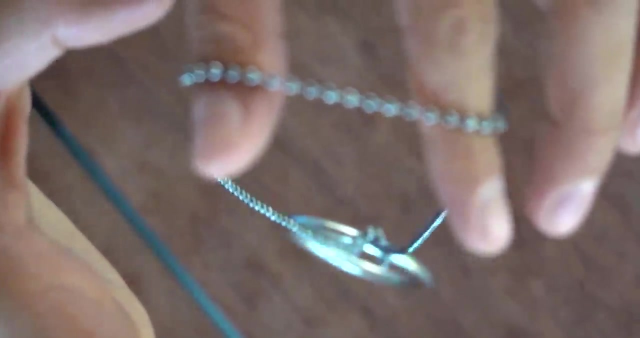 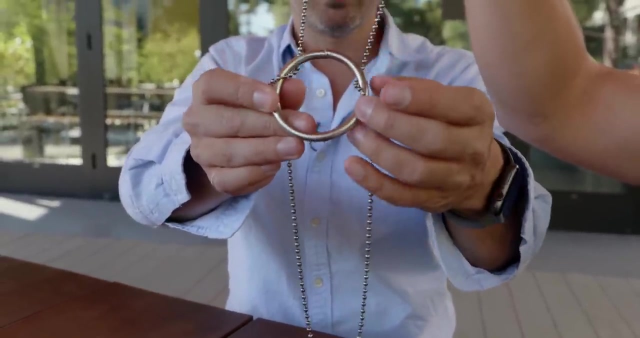 the ring will stick on the chain. It introduces just a little bit of rotation so that the ring rotates about 90 degrees and slides down the chain like this As it does, these pieces slide up the sides And when you get to the bottom, 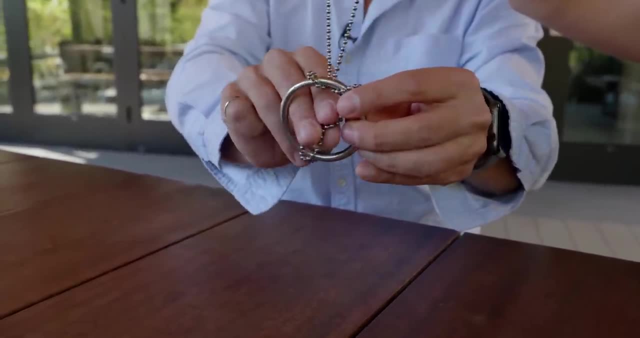 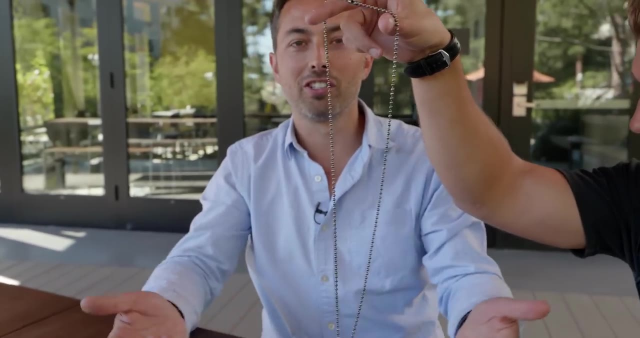 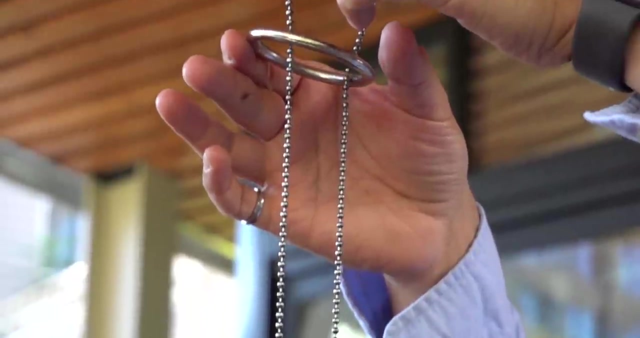 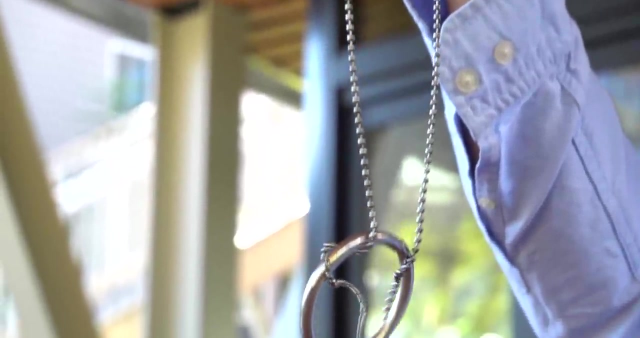 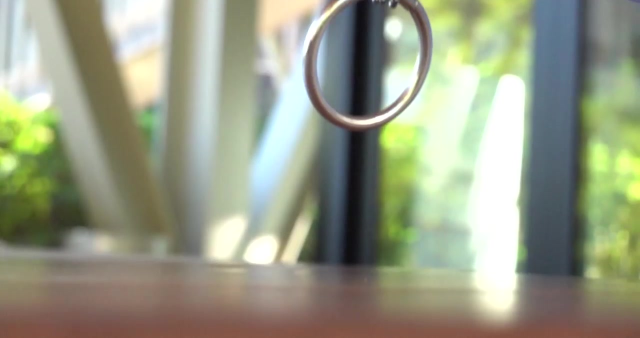 it's almost like this piece at the bottom gets sucked into the middle of the ring and then, at the last minute, gets pulled around and it snaps on and it's locked on like that. This is what it looks like. That's how you can get a ring locked onto a closed loop of chain. 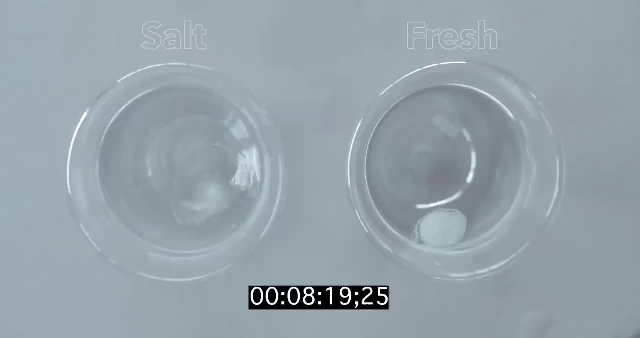 So back to problem number two. Why is the ice cube in fresh water melting faster than the one in salt water? Well, I think we can give it a little bit of a break- Okay, a better view of this- if I add a little bit of food coloring right on top of the ice cube. 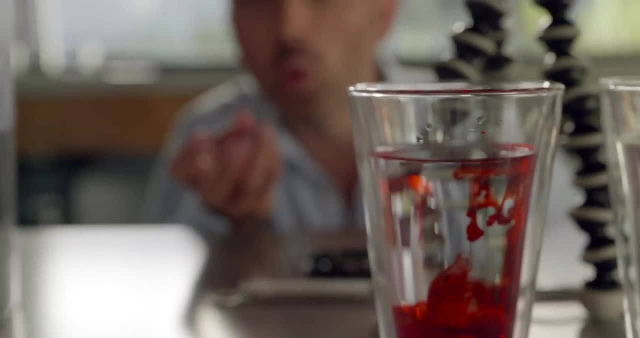 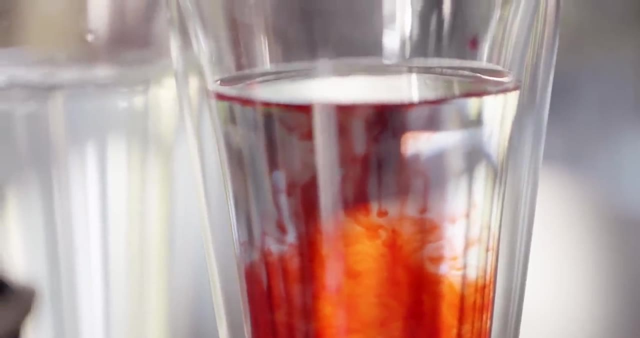 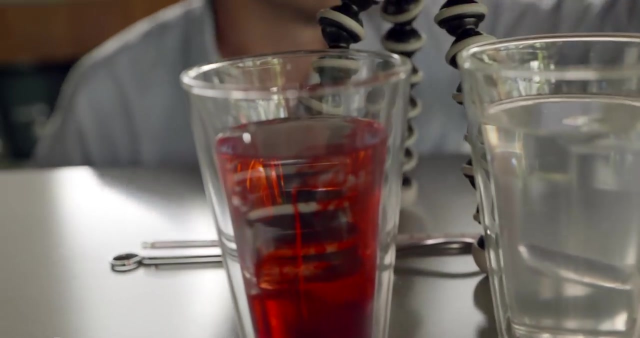 Because the water coming off that ice cube is cold, it's more dense than the surrounding fresh water and so it descends in the glass and that brings more warm, fresh water up to meet the ice cube, melting it faster, Whereas, on the other hand, in the salt water, as the ice cube melts, that fresh water is actually less dense than the salt water around it, and so it stays. that cold water that just melted off the ice cube stays around the ice cube, in effect insulating it from the warmer salt water around it. Okay, that seems like a very good idea. 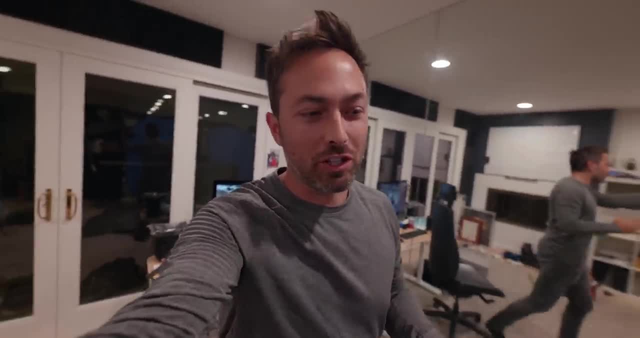 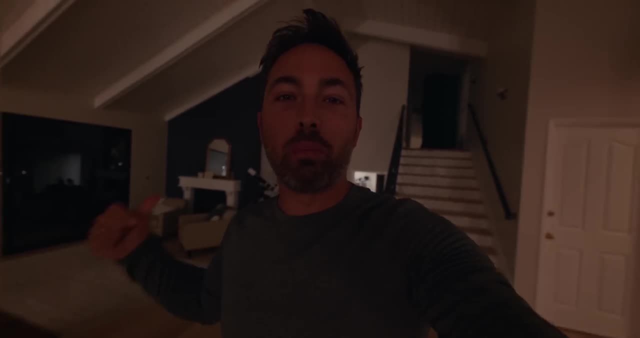 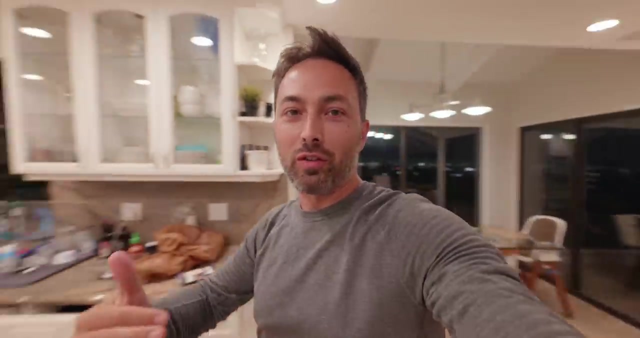 A very plausible explanation and maybe a convincing demonstration, but in the edit me from the future, I decided that, you know, maybe this wasn't the best way to explain this, because, well, you're just dropping food coloring in there and maybe food coloring would just float on the surface of salt water anyway and sink in fresh water. so not a good demonstration. 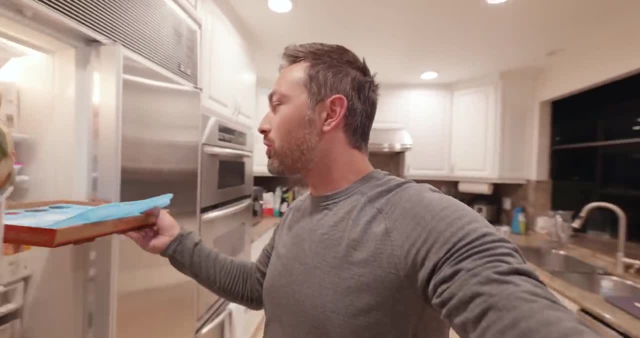 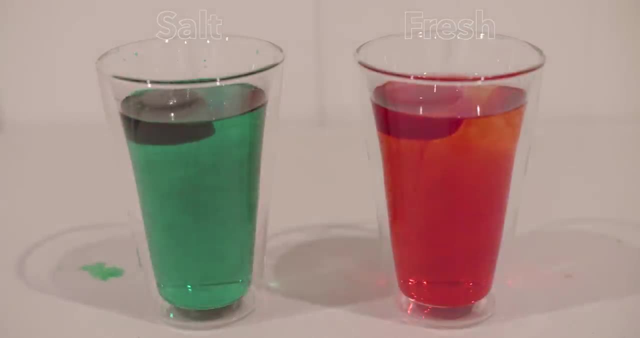 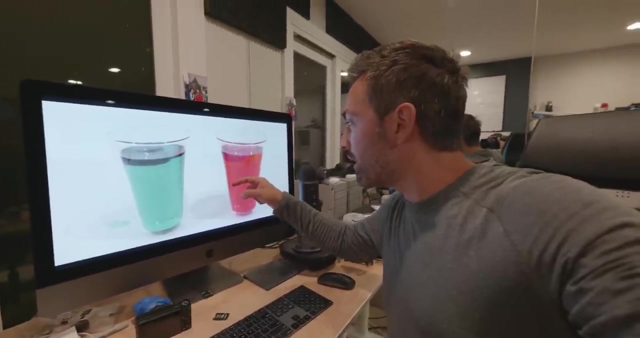 So a better demonstration I thought might be if we use colored ice cubes to begin with. Okay, I know there's a lot of food coloring in there and that makes things kind of hard to see, but I think you can clearly see the currents of cold water streaming down to the bottom of the cup. 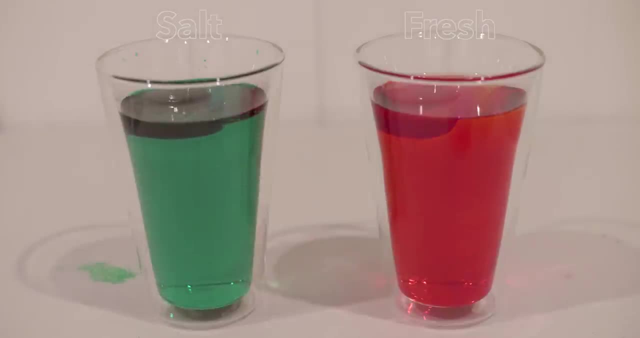 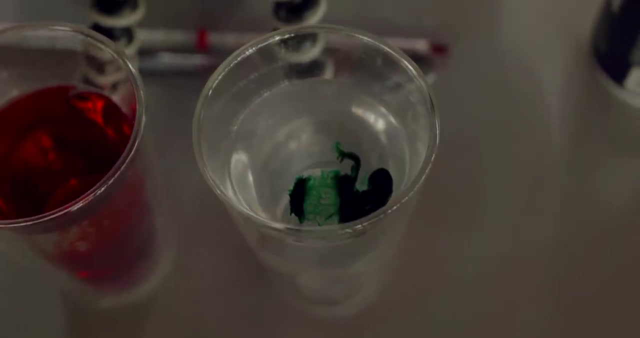 in the fresh water side and not in the salt water side. So I think this does clearly show what I was saying. The cool water that comes off the ice cube doesn't go down deep into the cup Over here. you can see, that's what's in there. 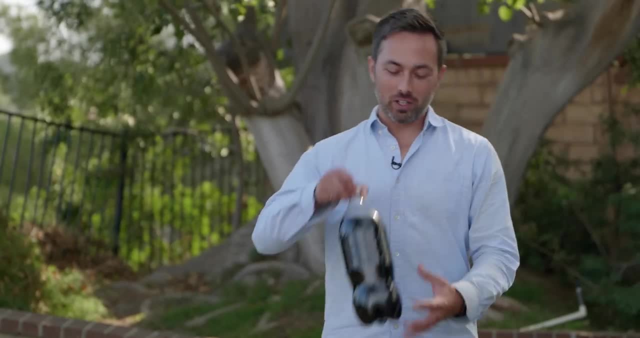 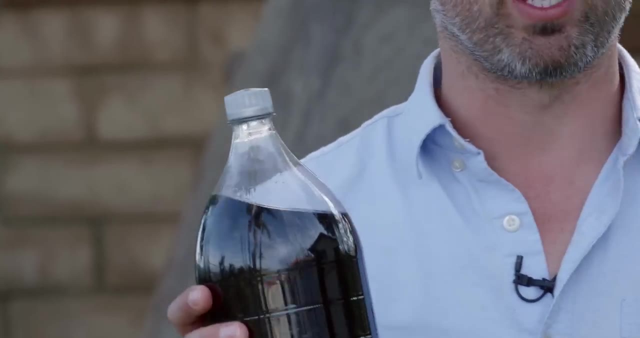 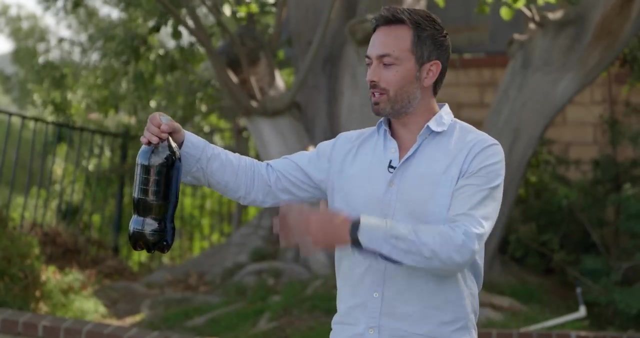 happened. so why do shaken carbonated drinks explode? first, let's explain why the pressure doesn't increase in the headspace when you shake it up. this is because of equilibrium. you know, when you pick up a bottle of soda in the grocery store, it's been sitting there for a few days. so the dissolved gas, the dissolved. 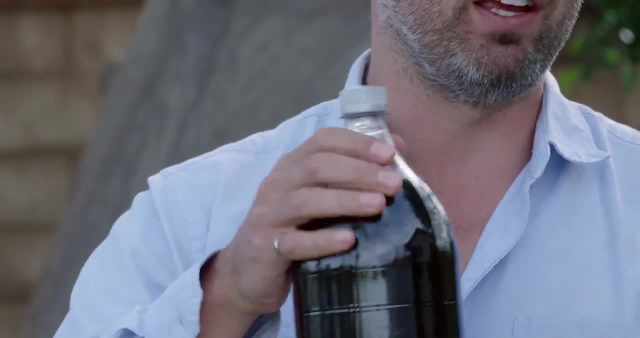 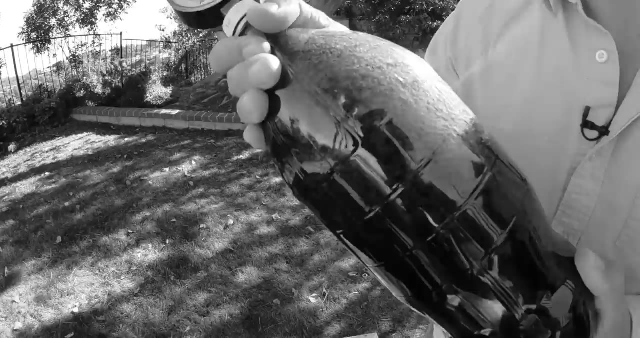 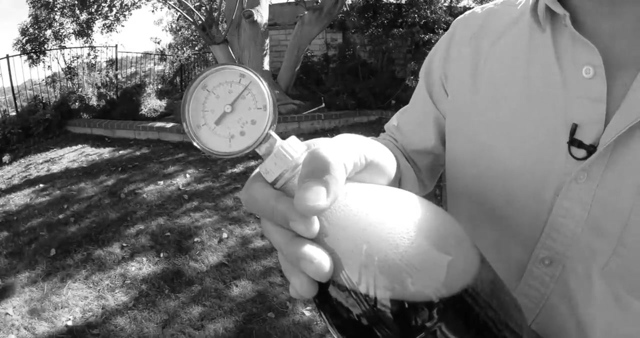 co2 in the liquid is at equilibrium with the gas up here in the headspace, and that equilibrium only depends on the temperature and the pressure of gas in the headspace. so no amount of shaking is going to change the pressure up here. for most soda bottles these days that pressure is about three atmospheres now. 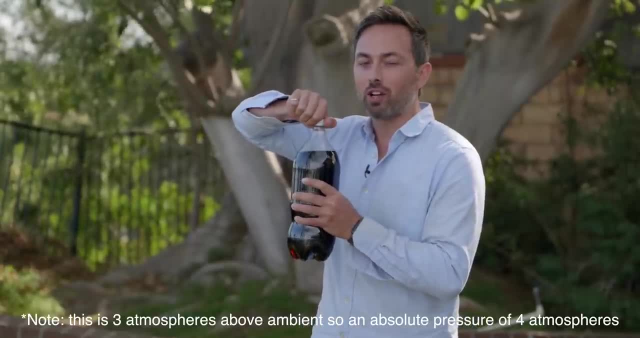 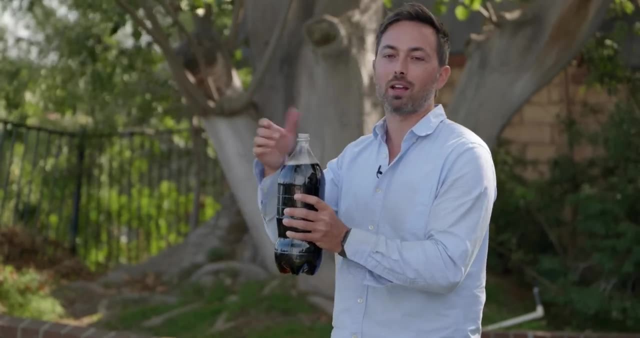 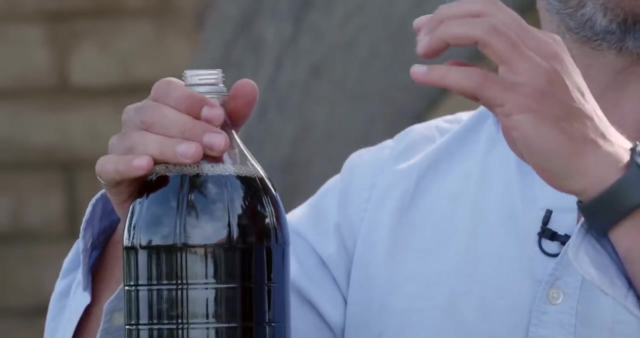 you can actually hear those three atmospheres of pressure get released when I open the bottle, but of course that's not messy, because it's just gas coming out the top. there's no liquid. but now the liquid is no longer in equilibrium. I mean it used to be under three atmospheres of pressure and now 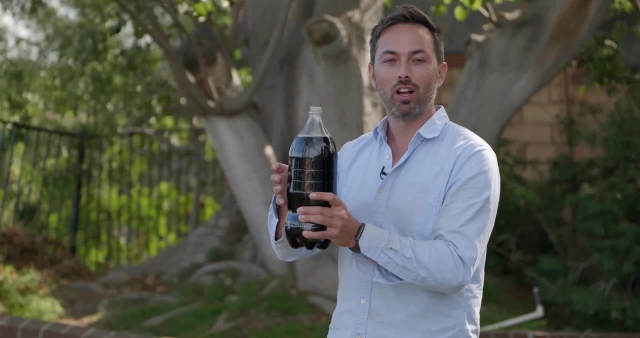 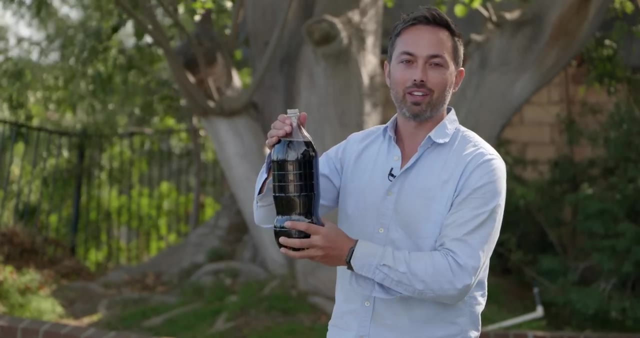 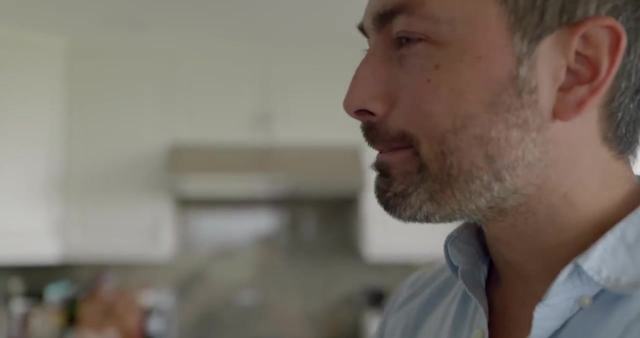 it's just under one atmosphere ambient pressure, and so because of that, there is more dissolved co2 in this liquid than would be at equilibrium at this pressure, and so the co2 starts to come out of solution. and well, those are the bubbles that you taste. that's why this drink is fizzy, non equilibrium beverage, and if 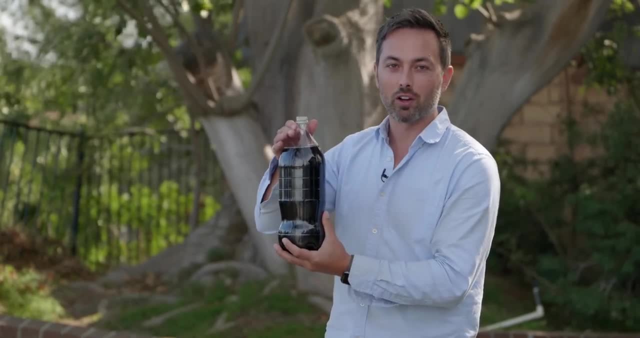 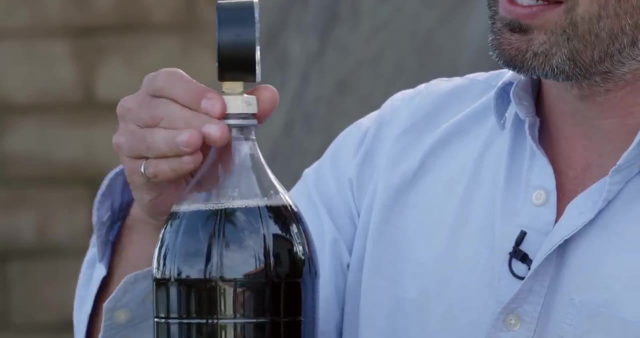 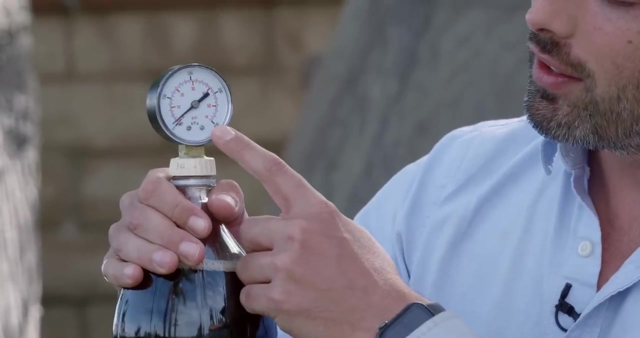 you leave it open, those bubbles will keep coming out until the whole drink goes flat. I'm going to put the pressure gauge on top of this bottle so we can actually see the co2 coming out of solution and increasing the pressure right here. and if I left this bottle alone for long enough, the pressure would eventually. 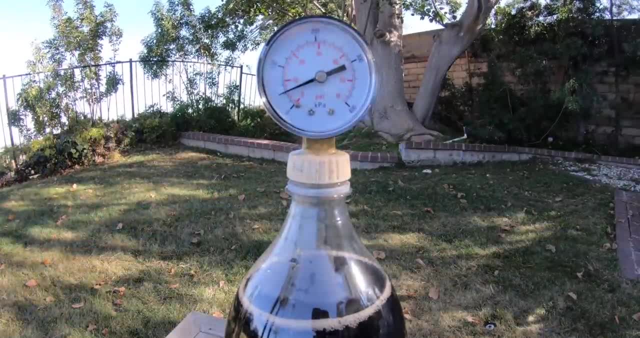 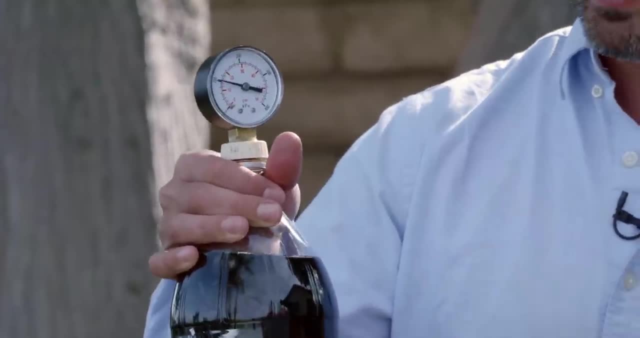 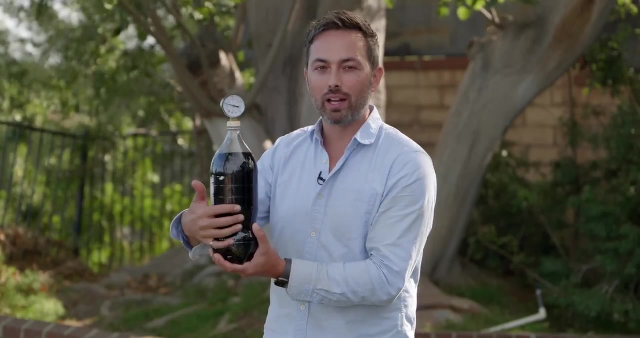 come back to equilibrium three atmospheres. but as you can see, it is a very slow process and that's because it's actually quite hard for dissolved gas like co2 to spontaneously come out of solution. so what we can accelerate this process is by introducing nucleation sites into 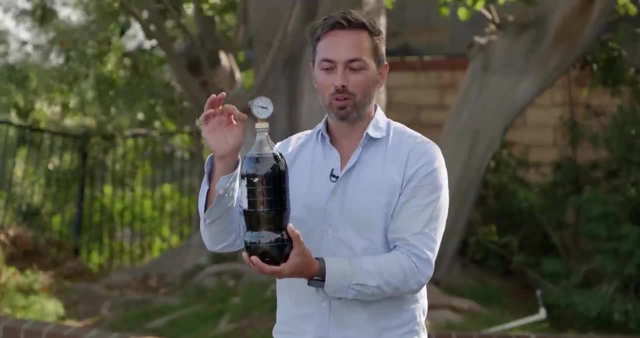 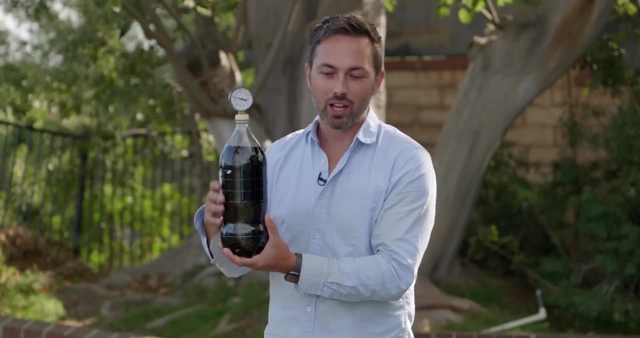 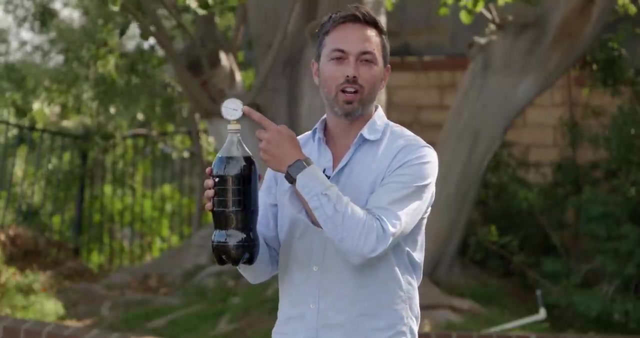 the liquid, and one example of a nucleation site is a tiny gas bubble. so if I shake up the bottle, what I'm actually doing is introducing little nucleation sites, tiny air bubbles, into the liquid, and that makes it easier for the co2 to come out of solution, and so we'll see this pressure increase much. 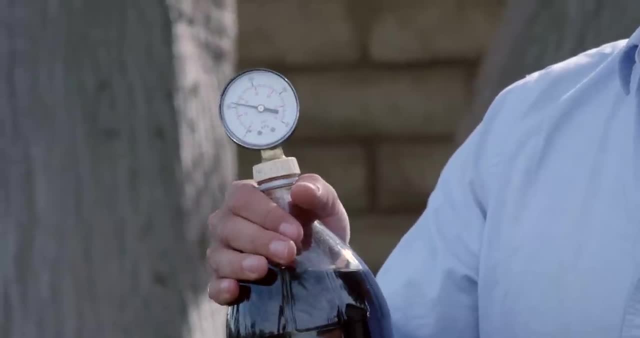 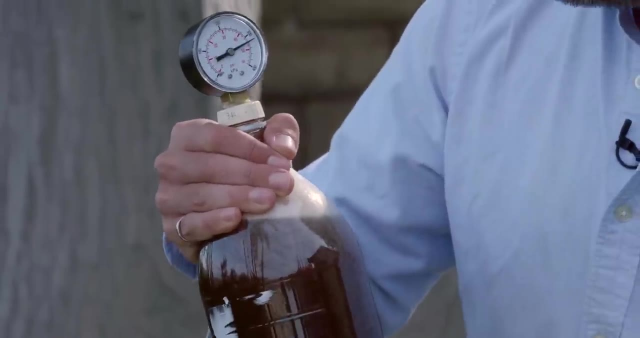 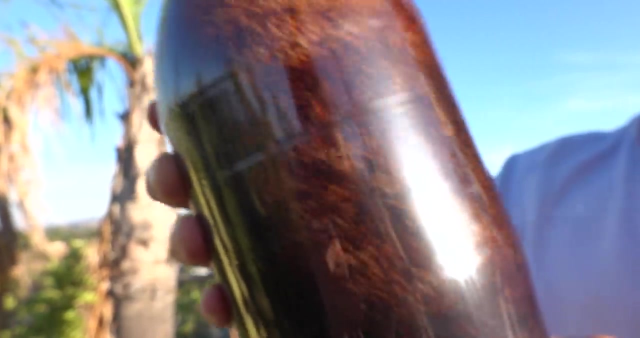 more rapidly. you ready? I'm gonna shake it up in three, two, one. and there you see, the pressure has quite quickly come back to about three atmospheres, 320 kilopascals. so if you shake up a closed carbonated drink that's been at equilibrium well, you are not increasing the pressure in the 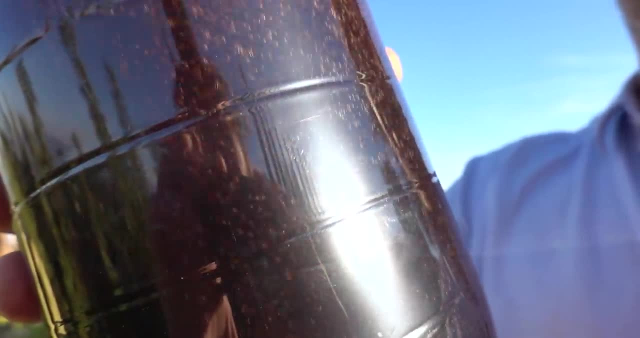 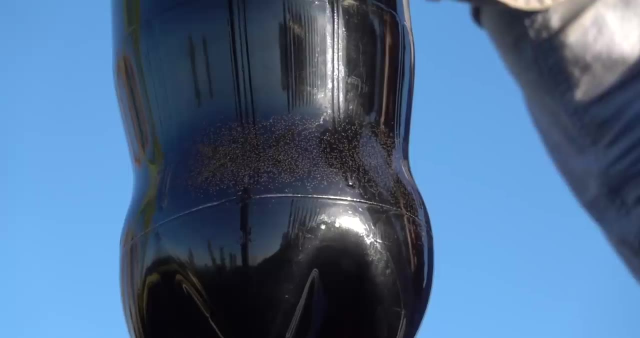 bottle. but you are introducing tiny air bubbles into the liquid which act as nucleation sites. some of them cling to the walls of the bottle. so when you go to open it, those bubbles do two things. first, they expand due to the decrease in pressure, and that pushes up the liquid. 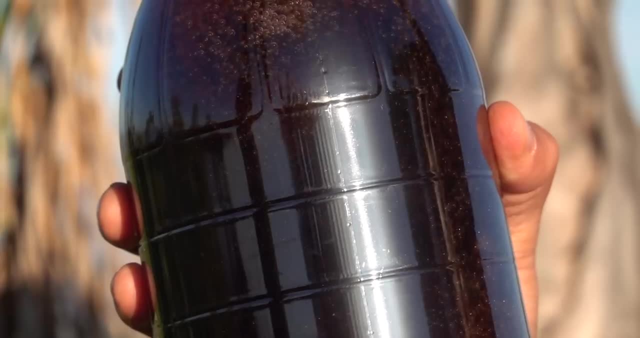 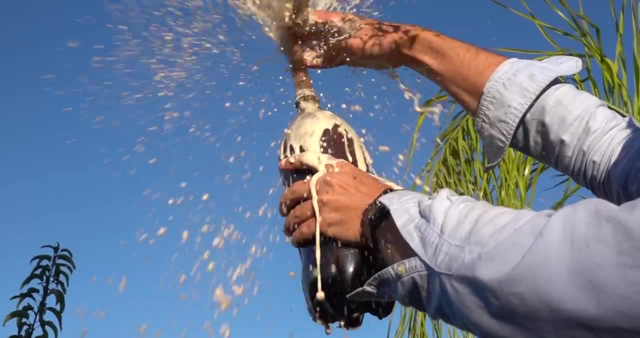 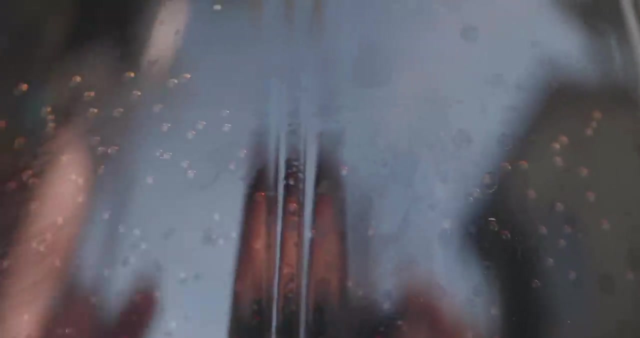 above them, and second, they act as nucleation sites, allowing the dissolved co2 to come out of solution much more rapidly, and so that's what leads to the carbonated drink explosion. but this suggests a way to disarm a shaken carbonated beverage, and that is by flicking the walls of the bottle. that 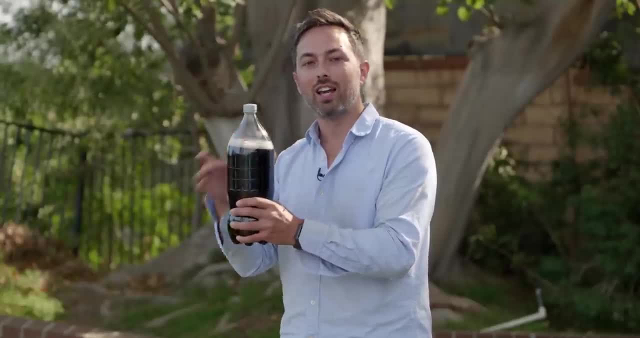 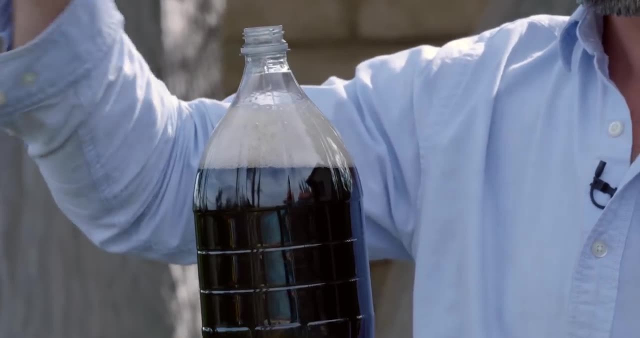 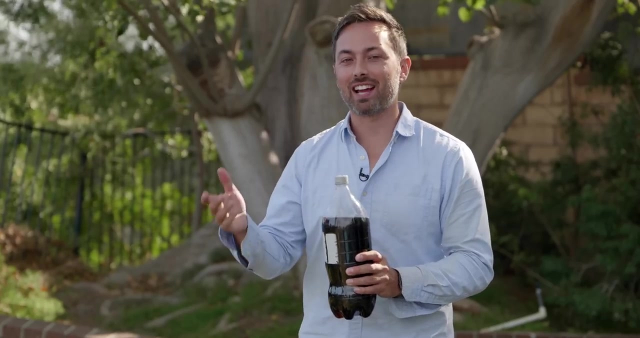 gets rid of those bubbles that are clinging to the sides and allows you to open the bottle without incident. huh, it worked. now is there a way to introduce nucleation sites into a carbonated drink without shaking it? yes, that's exactly what you're doing when you 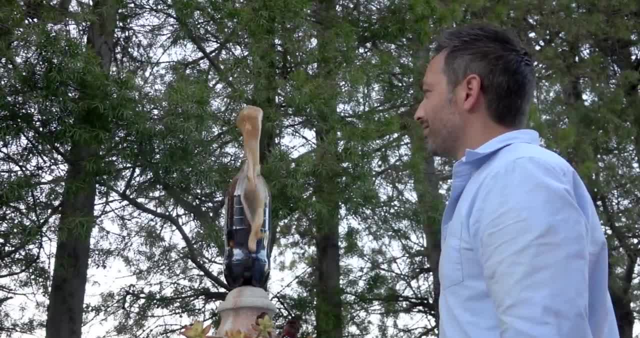 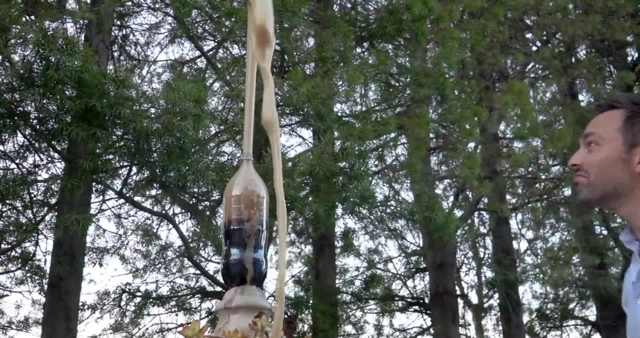 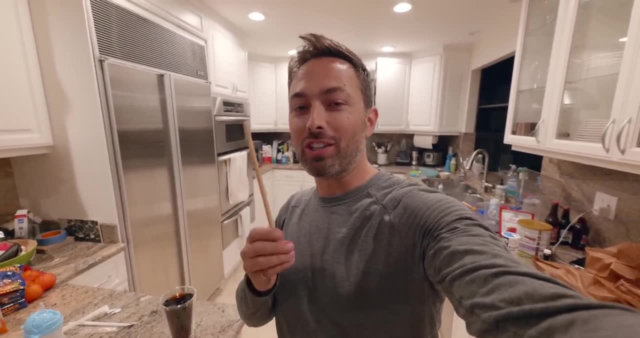 put a Mentos in a carbonated drink. the rough surface of the Mentos acts as a nucleation site which allows the co2 to come out of solution much faster, creating the soda fountain me again. so when I showed this video to Diana, the physics girl, she asked whether paper straws have more nucleation sites than 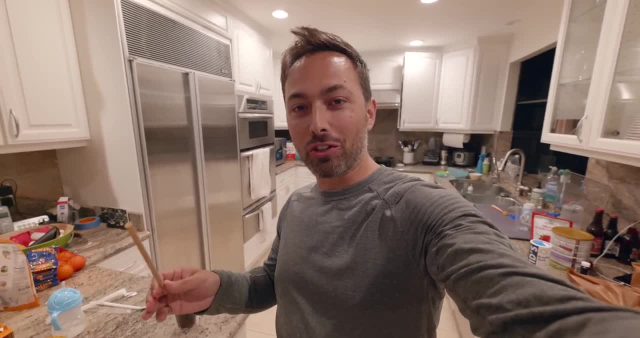 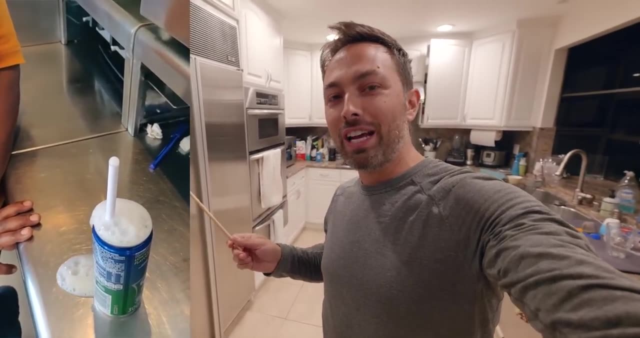 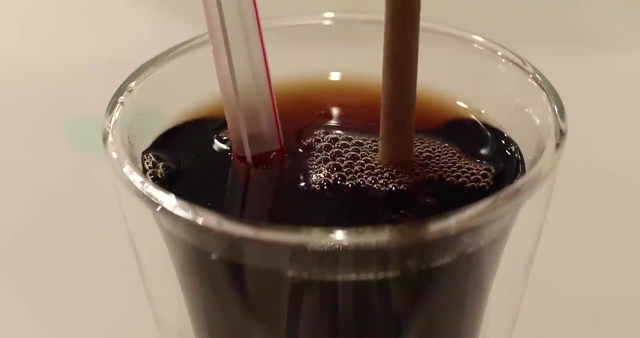 plastic ones and, to be honest, I'm not sure about the research around this, but there are some other YouTube videos showing how drinks overflow when you put a paper straw in, and also my little preliminary analysis with this paper straw show that it does indeed create more bubbles than a plastic straw. so if 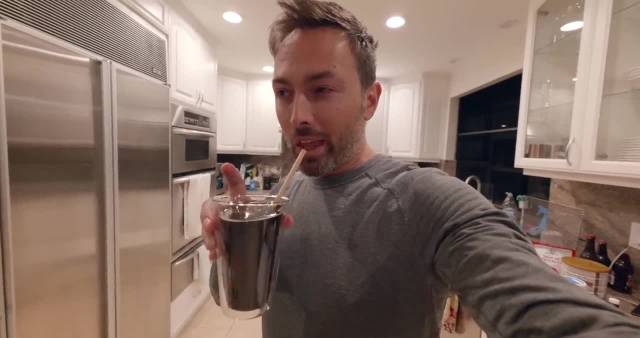 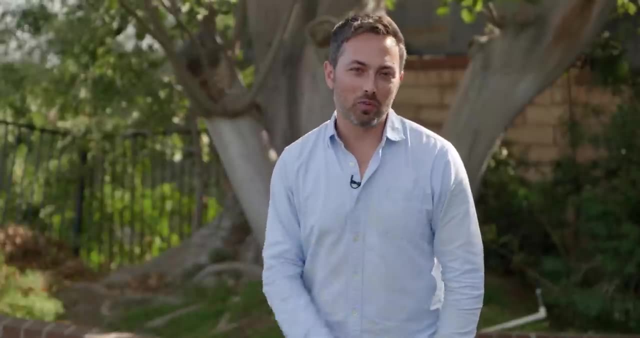 you needed another reason to hate paper straws. well, there you go. they make your carbonated drink more fizzy as it comes up the bottom of the bottle, and that's why I'm doing this video today: the straw. this has been three perplexing physics problems. if you have any other, 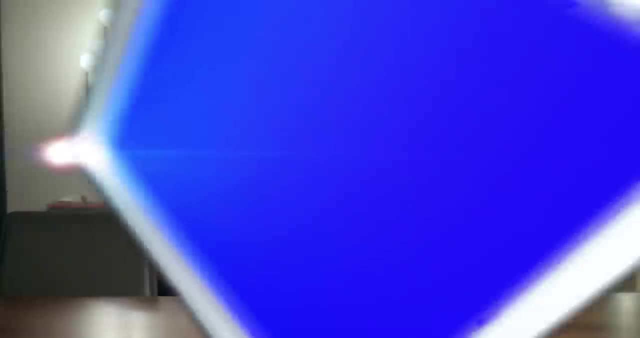 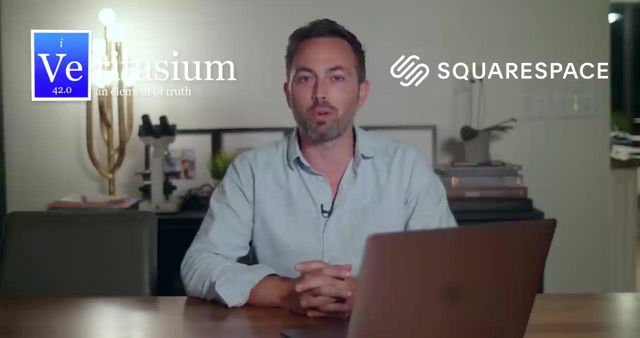 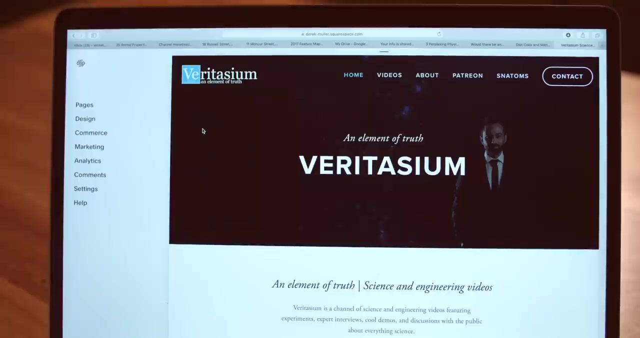 perplexing science problems. put them in the comments below. hey, this portion of the video is sponsored by Squarespace, the all-in-one platform for building a professional website, online store or portfolio. in fact, about a year ago, I remade my website veritasiumcom on Squarespace and I found it so much. 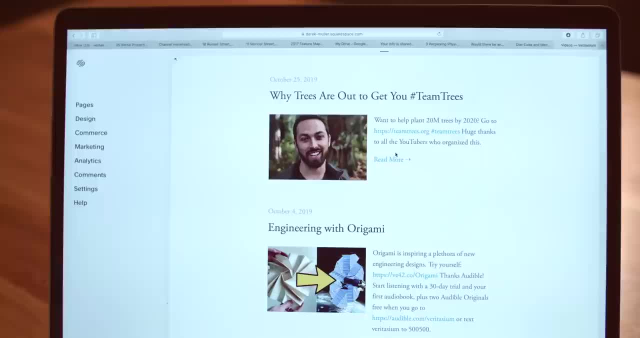 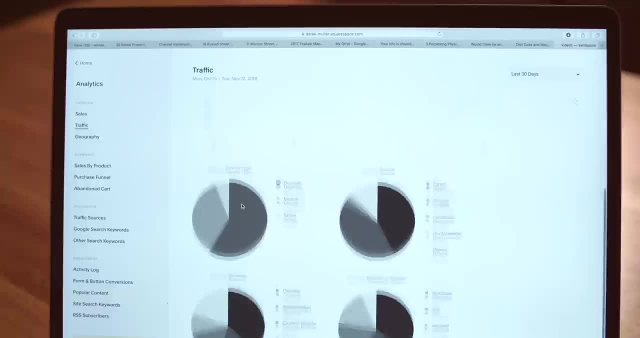 quicker, easier and cheaper than going through a web developer, who I always had to contact in order to make changes. Squarespace gives me great analytics so I can see who's coming to the site and when, from where, and what they're spending the most time on, and that allows me to see. 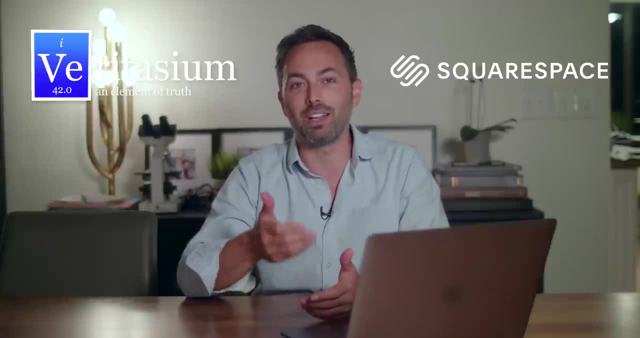 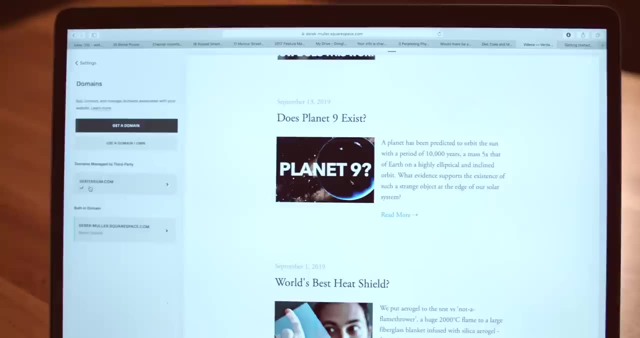 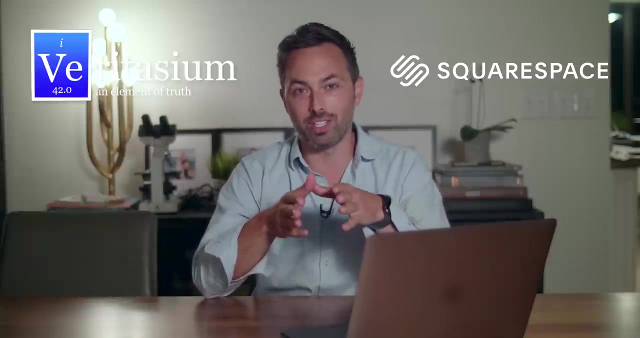 what people are really enjoying, which helps me decide what to make next. now, if you're just getting started, well, you can purchase your domain directly through Squarespace, which saves you the hassle of setting up domain name servers and all that kind of stuff. plus, each domain comes with free Whois privacy, because 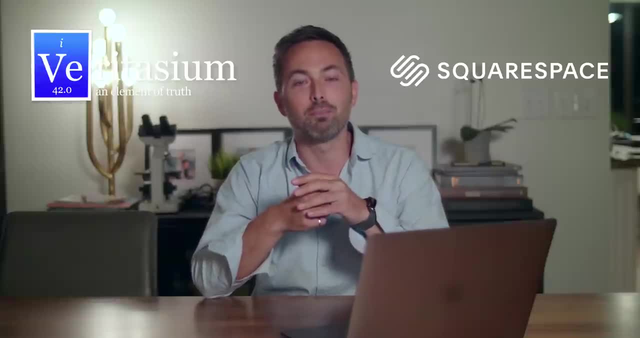 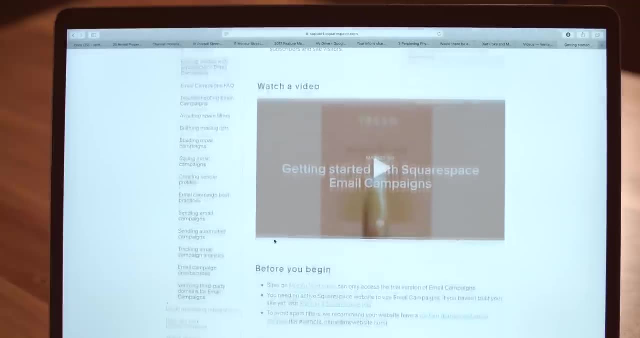 nobody wants a domain that reveals all your details. and if you want to run email campaigns, Squarespace can do that, making the look and feel of all your communications consistent. or how about an online store? Squarespace can do that, too, with e-commerce templates, inventory management.